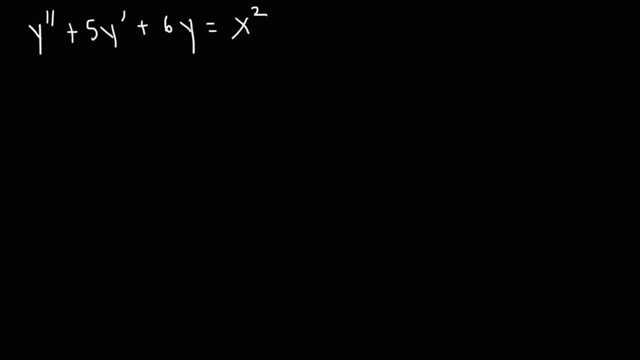 Now, this particular equation is a non-homogenous differential equation. It's in the form ay prime, I mean ay double prime plus by prime plus cy is equal to g of x. Since g of x is not zero because it's x squared, we have a homogeneous, I mean a non-homogeneous. 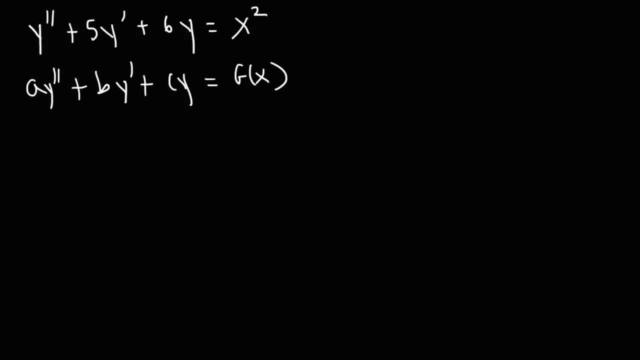 or non-homogenous differential equation. To find the general equation we're going to need to find the general equation. We're going to need to find the general equation. To find the general solution. we need to use this formula: y of x is going to equal y sub p of x plus y sub c of x. 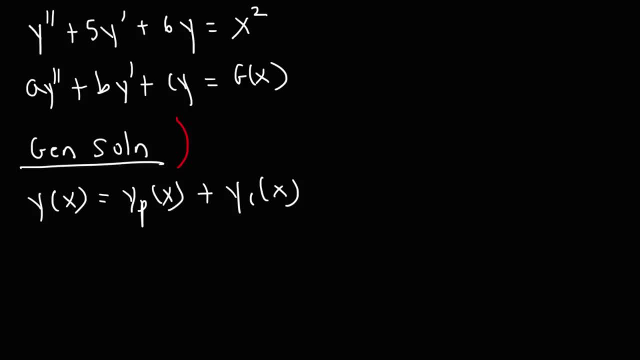 Now y sub p of x. that is the particular solution of the non-homogeneous differential equation. Now there's another equation that we need to talk about, And it is the homogenous differential equation in the form: ay prime, y prime plus- by prime I mean ay double prime plus by prime plus cy is equal to zero. 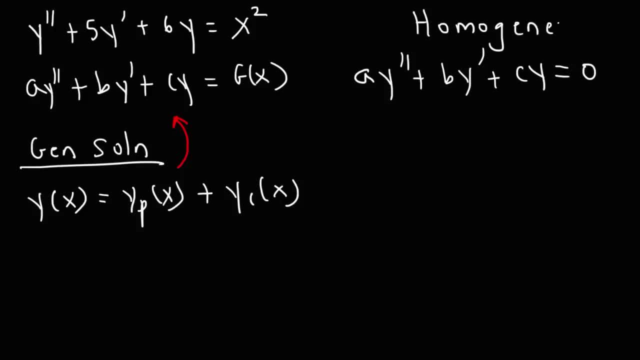 So that is the homogenous differential equation, since we can see that g of x is zero. Now solving the homogenous equation will give us y of c. Combining those two will give us the general solution to our original non-homogenous differential equation. 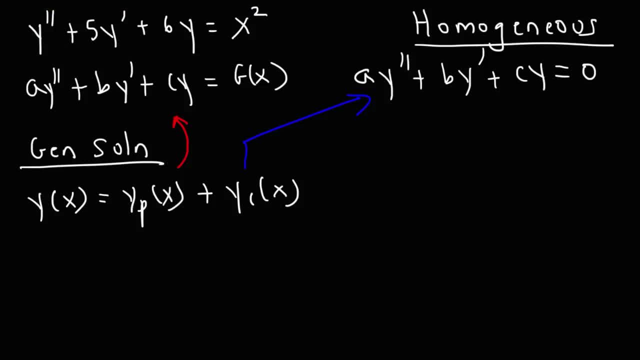 So I'm going to talk about how we can do everything, But for now, just make sure you have these three equations. By the way, this video builds on another video that I created entitled Second Order- Linear Differential Equations, which explains how to solve homogenous differential equations. 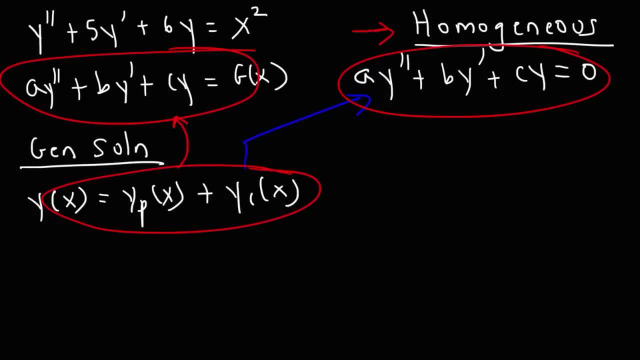 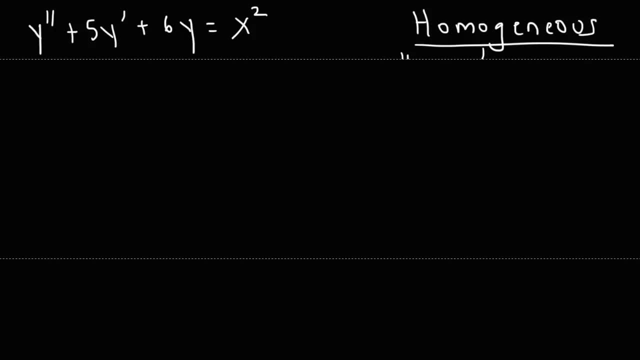 You may want to watch that video, if you haven't done so already, before continuing to watch this one. So let's go ahead and continue. Let's continue with this problem Now. the first thing that we're going to do is solve the homogenous differential equation where g is equal to zero. 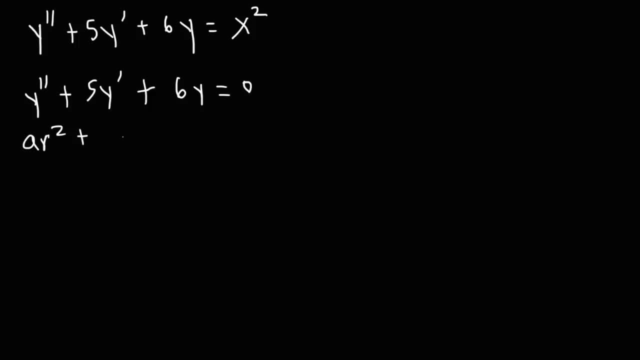 So we have this auxiliary equation: ar squared plus br plus c is equal to zero. So we can see that a is 1., b is 5.. c is 6.. To factor this trinomial we need two numbers that multiply to 6, but add to the middle coefficient 5.. 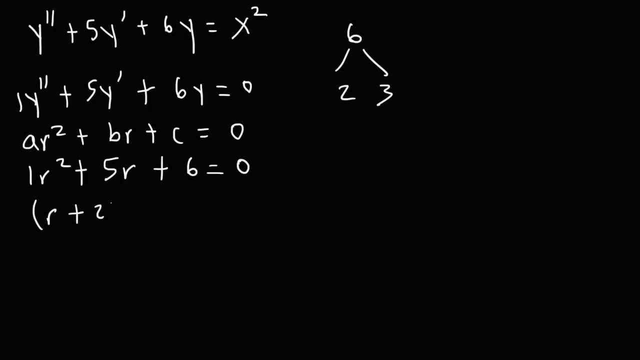 So that's going to be 2 and 3. So we can factor it as r plus 2 times r plus 3.. And so we get r is equal to negative 2 and r is equal to minus 3.. 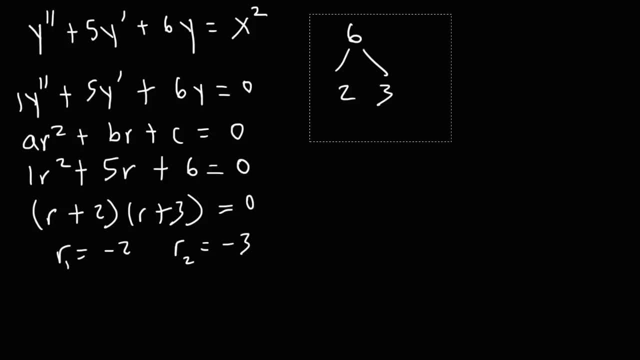 So we have two real solutions, which means we're dealing with case number 2 of solving our homogenous differential equation. So the general solution is going to be c1e- r1x plus c2e- r2x- r1 is minus 2.. 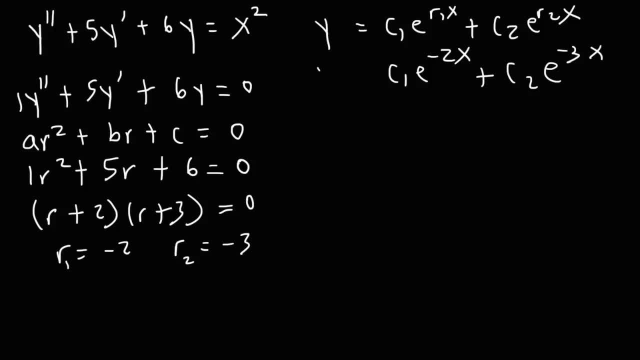 r2 is negative 3. And so this is going to be y sub c. So that gives us the general solution of our complementary equation. So I'm going to write that on the bottom, Because we're going to need that later. 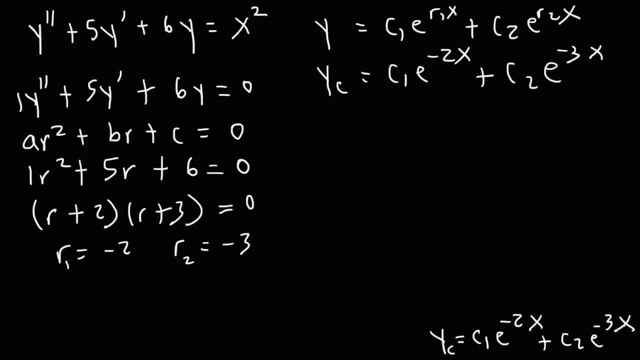 So let's save this for the end. Now the next thing we need to consider is g. g is equal to x squared, And so y must equal a polynomial of degree 2. So therefore, y sub p of x will have the general form ax squared plus bx plus c. 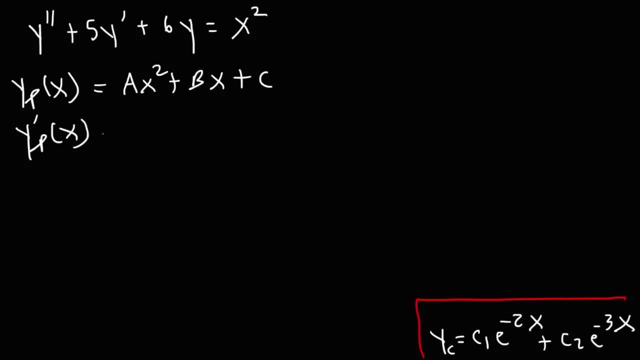 If we take the first derivative of that, we get this: The derivative of x squared is 2x, So this is going to be 2ax. The derivative of x is 1.. So we get b. Now finding the second derivative of y sub p is just going to be 2 times a. 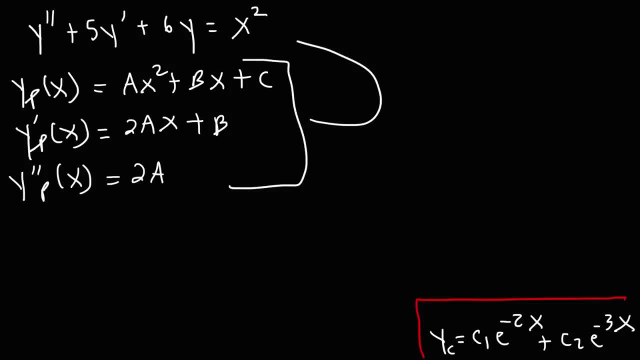 Now we're going to take all of this information and plug it in to that function, So we can replace y double prime with 2a And then y prime with 2ax plus b, And y is going to be replaced with ax squared plus bx plus c. 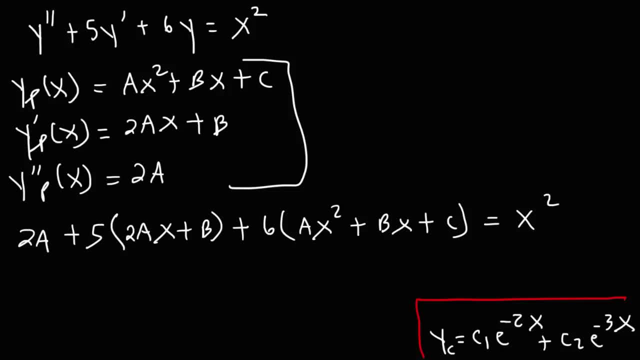 And so this is going to equal x squared. Now we're going to take all of this information and plug it in to that function. Now what we need to do is solve for a, b and c. So let's distribute. 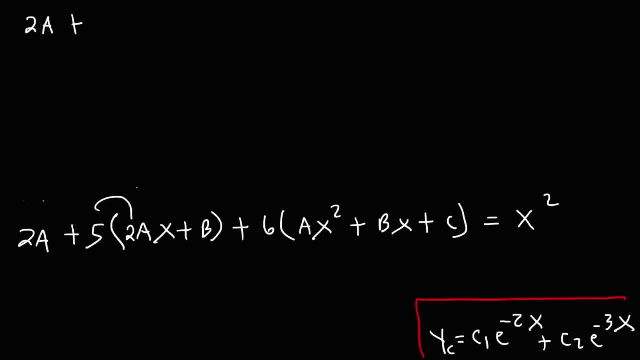 So we have 2a plus That's going to be 10ax, And then plus 5b. Distributing the 6 is going to be 6ax squared Plus 6bx plus 6c is equal to x squared. 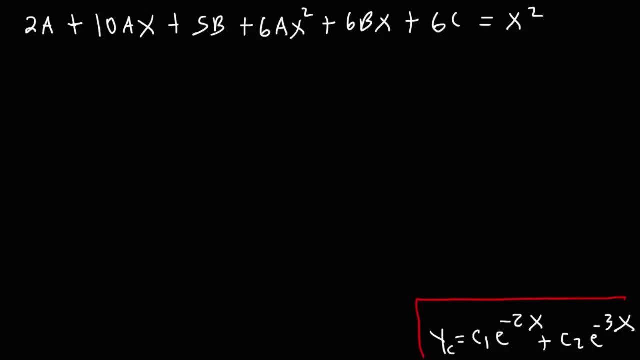 There's only one term with an x squared on the left, So I'm going to write that as 6a times x squared. Now there are two terms on the left with an x variable, So I'm going to factor out the x. 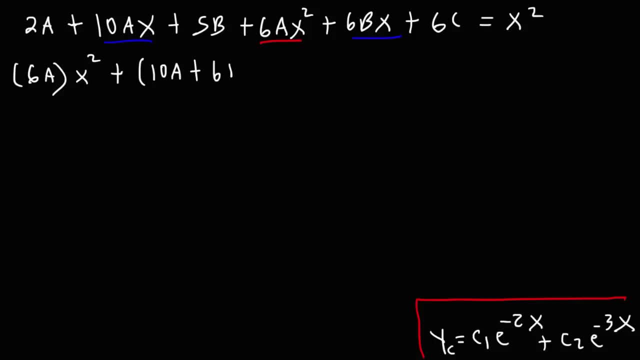 And I'm going to have 10a plus 6b times x, And then we have three constants, Which I'm going to write it as 2a plus 5b plus 6c, And so this is going to equal 1x squared plus 0x plus 0.. 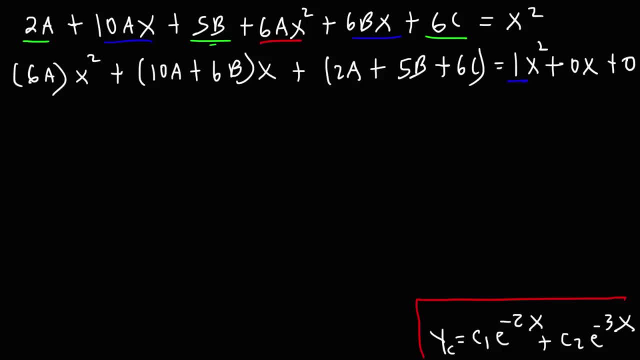 So the coefficient on the right side in front of x squared, is a 1.. On the left it's a 6a, So we can set those two equal to each other. So 6a is 1.. Divide them both sides by 6.. 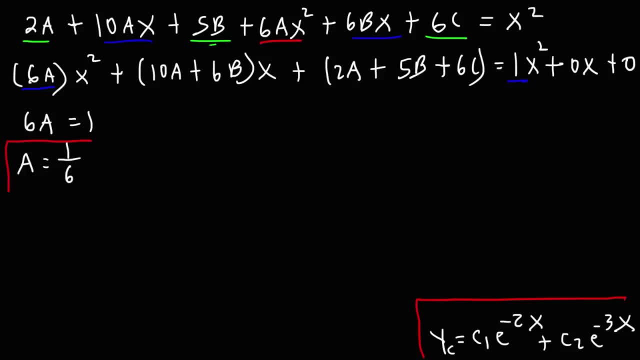 We can see that a is 1 over 6.. So that's our first Coefficient. Now let's move on to the next one. So the coefficient in front of x is 10a plus 6b, And that has to equal 0.. 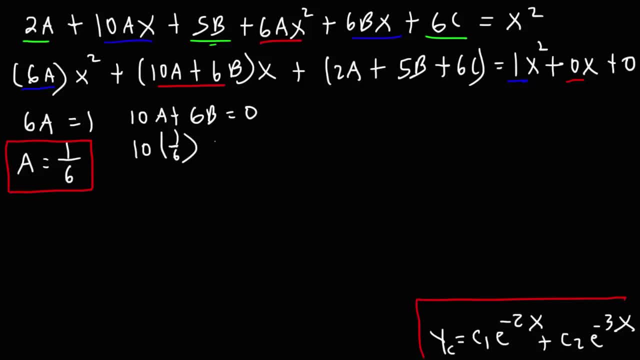 Replace an a with 1 over 6.. We have this. Now. to get rid of the fraction, I'm going to multiply everything by 6.. 10 times 1 over 6 times 6 is simply 10.. And then 6b times 6 is. 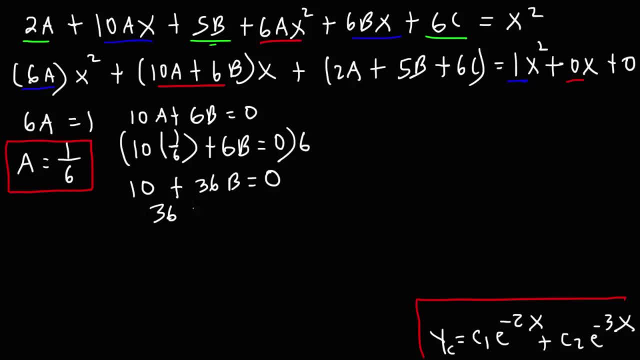 36b. So we have 36b is equal to negative 10.. Divide them both sides by that, We get negative 10 over 36.. Reducing that fraction, Half of 10 is 5.. Half of 36 is 18.. 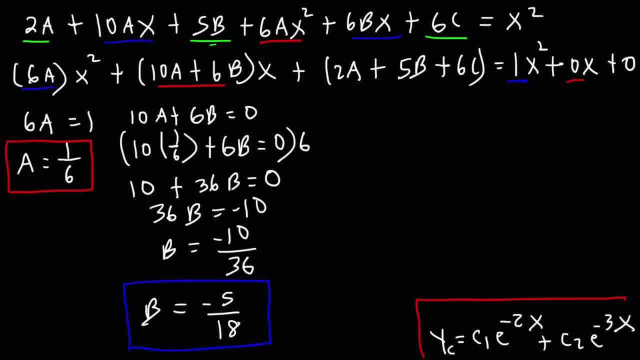 So b is negative 5 over 18.. Now for the next one. this must equal 0. So we have 2a plus 5b plus 6c equals 0. So we're going to replace a with 1 over 6 and b with negative 5 over 18.. 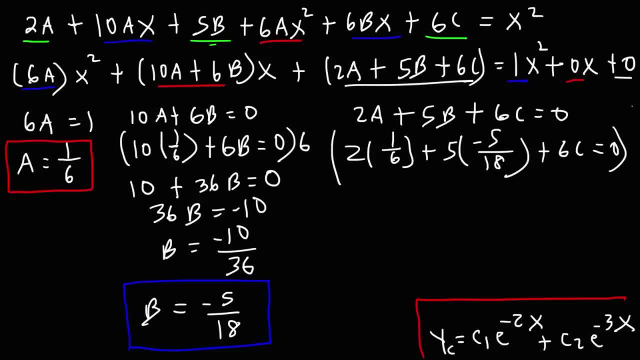 And let's solve for c. So to get rid of both, or the two fractions that we have, let's multiply everything by 18.. 18 divided by 6 is 3 times 2. That's 6.. Here the 18s will cancel. 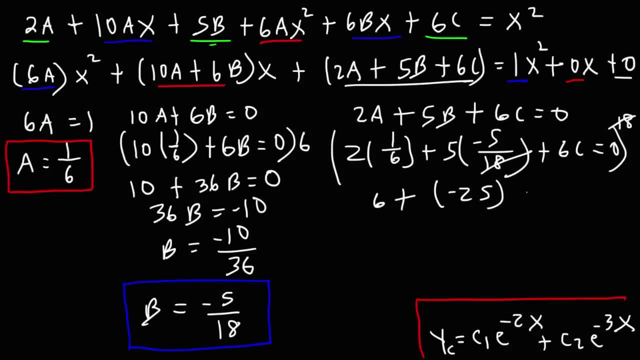 So we have 5 times negative 5.. That's negative 25.. And then 6 times 18.. That's going to be 108.. 6 minus 25 is negative 19.. So, moving out to the other side, we have 108c is equal to 19.. 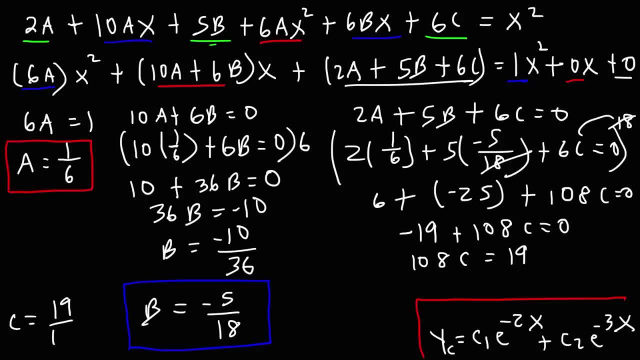 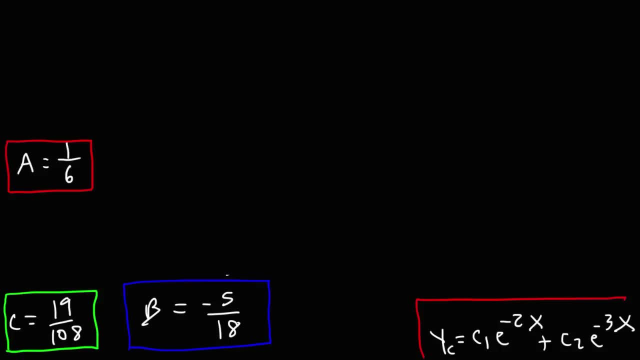 So c is 19 over 108.. So now that we have the values of a, b and c, We can now write our answer. So we said that y sub p of x is in the form ax squared plus bx plus c. 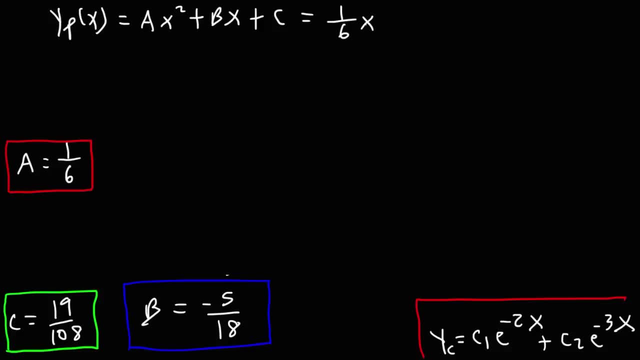 So substituting those in, it's going to be 1 over 6x squared, minus 5 over 18x, plus 19 over 108.. Now the general solution to the non-homogeneous differential equation is going to be y sub c plus y sub p. 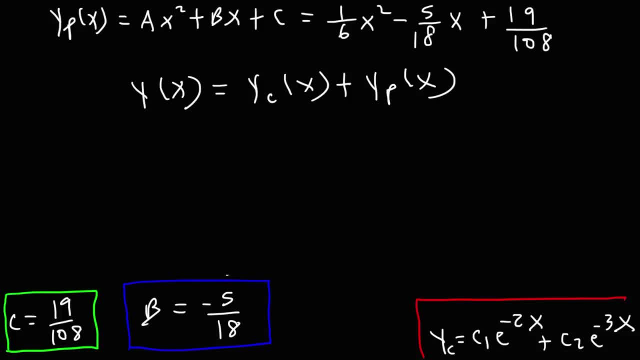 So now, this is when we're going to put everything together. So let's start with y sub c, which we have right here. So that's c1 e to the negative 2x plus c2 e to the negative 2x. 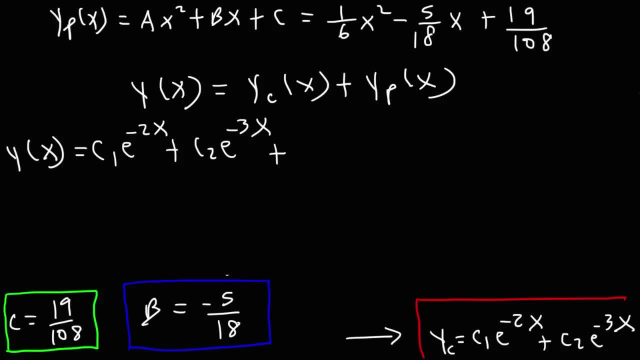 Next we need to add y sub p, which is what we have here. So that's plus 1 over 6x, squared minus 5 over 18x, plus 19 over 108.. So this, right here, is the solution to the non-homogeneous second order linear differential equation. 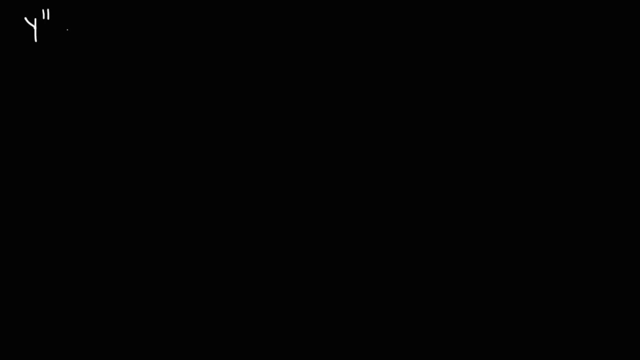 Now let's move on to the next example. Let's say we have y double prime Plus 9y, And let's say that's equal to e to the 2x. Go ahead and solve this differential equation. So first let's write the homogeneous differential equation where g of x is equal to 0.. 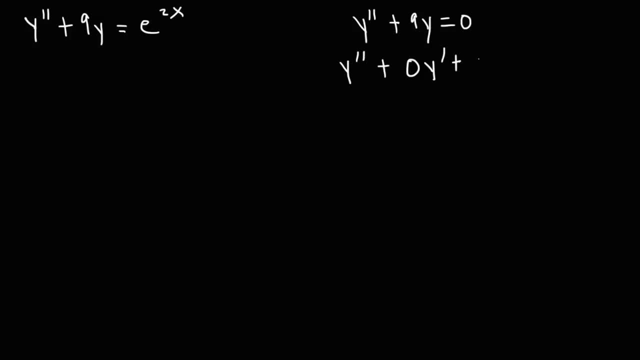 Now keep in mind we're missing 0y squared, So I'm going to write it here. So now we need to determine the values of a, b and c, So we can see that a is 1, b is 0,, c is 9.. 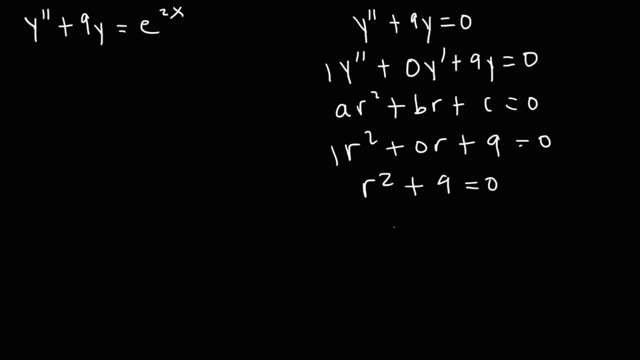 So we have r squared plus 9 is equal to 0.. Moving the 9 to the other side, we have this: Taking the square root of both sides, r is plus or minus 3i. So r1 is going to be 0 plus 3i. 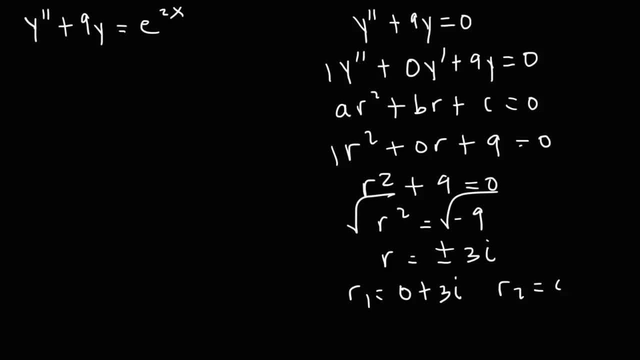 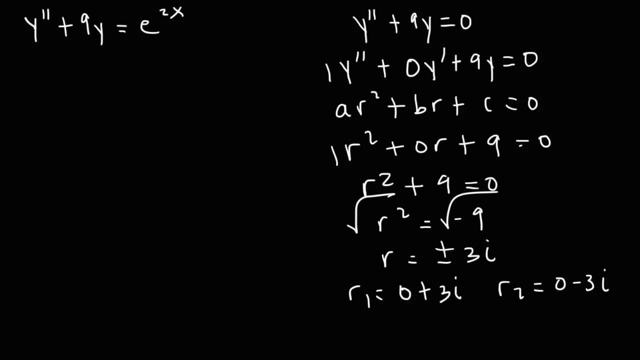 So for this homogeneous differential equation we have two imaginary solutions. So this is case number 3.. So keep in mind: r1 is equal to alpha plus beta i, So we can see that alpha is equal to 0 and beta is equal to 3.. 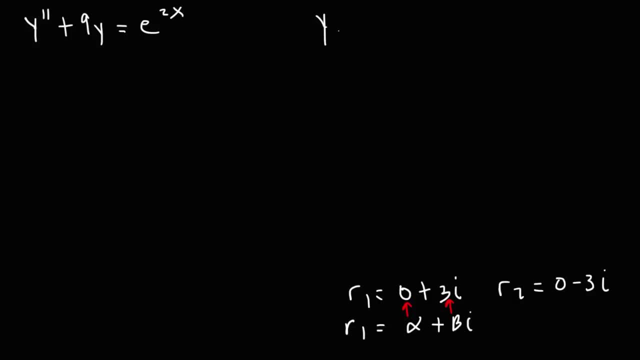 So the general form of our complementary equation, the general solution rather, is going to be: for case number 3, it's e alpha x times c1, cosine beta x plus c2 sine beta x, Now alpha is equal to 0.. 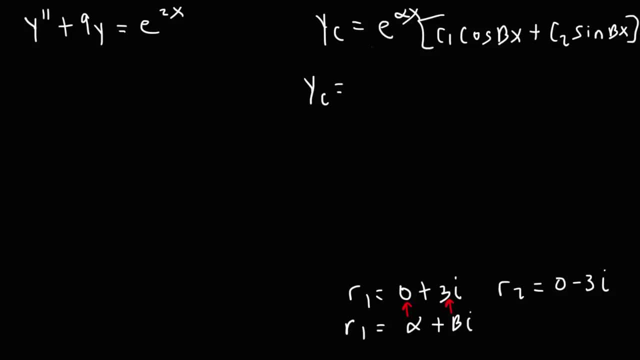 And e to the 0 is 0. So this part basically disappears And we're going to have c1, cosine beta x, but beta is 3. So cosine 3x And then plus c2 sine 3x. 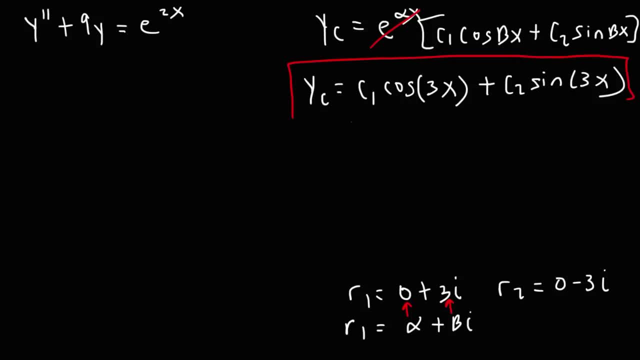 So we're going to save this equation for later. So that's the general solution of the complementary equation. Now let's focus on our original equation. So let's focus on our original equation. Notice that g is e to the 2x. 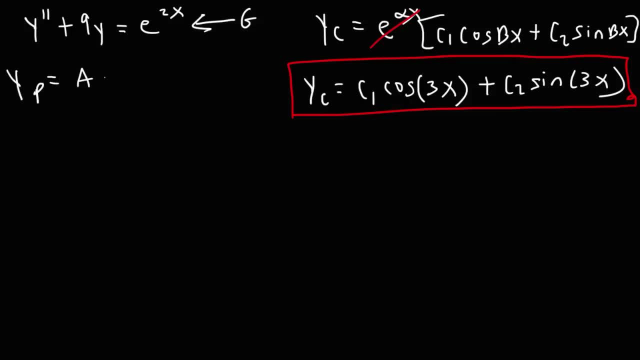 So yp is going to have the general form ae to the 2x. Our next step is to find the first derivative of that. The derivative of e to the 2x is going to be: it's e to the 2x times the derivative of 2x, which is 2.. 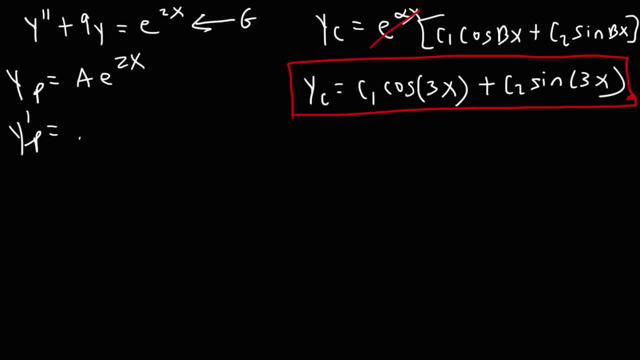 So we can write that as 2a e to the 2x. Now to get the second derivative, it's going to be 4a e to the 2x if you follow the same process. Now our next step is to take all of this and plug it in to the original expression. 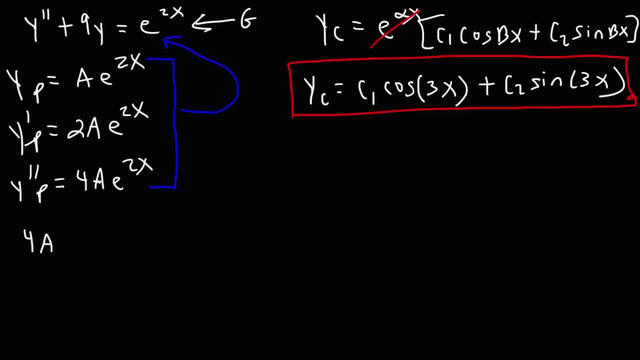 So replace in y double prime with 4a e to the 2x, and then we're going to replace y with a e to the 2x and that's going to equal g. So these two are like terms. 4a plus 9a will give us 13a e to the 2x. 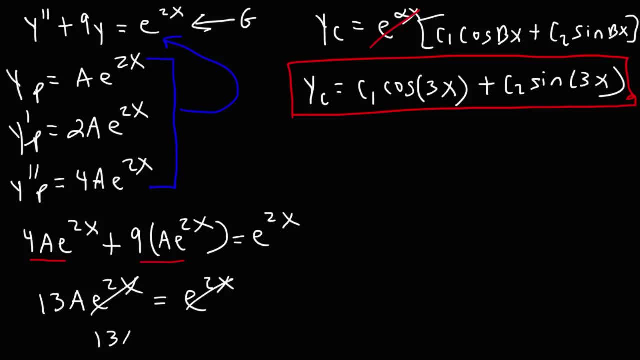 So we could divide both sides by e to the 2x and we'll get: 13a is equal to 1.. So a is 1 over 13.. Taking this and plugging it into that expression, we get yp is equal to 1 over 13. 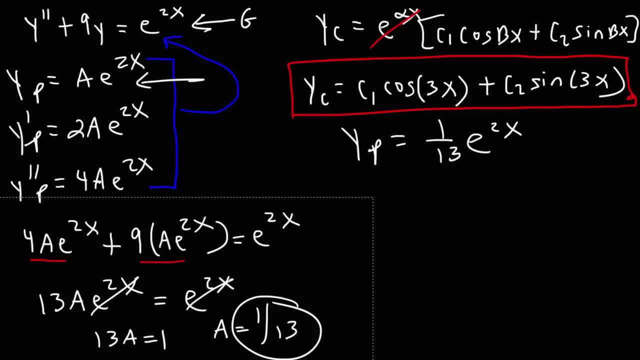 e to the 2x. So we're going to divide both sides by e to the 2x and we'll get: 13a is equal to 1 over 13.. e to the 2x. So now we have everything we need to write the final solution. So it's going to be yc plus yp. 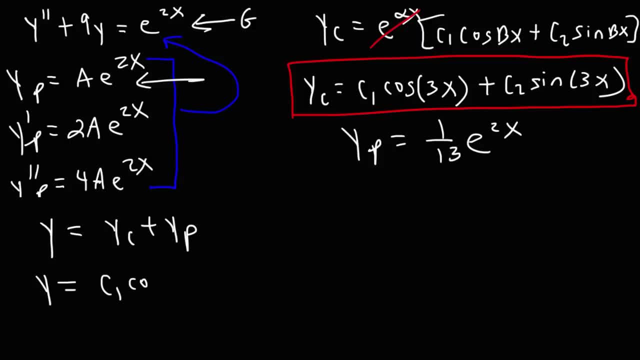 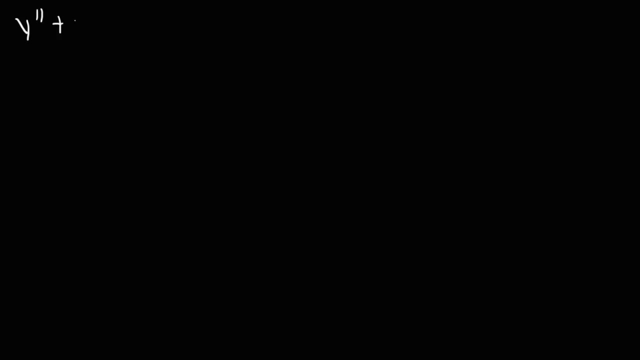 which is c1 cosine 3x plus c2 sine 3x, and then plus yp, which is 1 over 13 e to the 2x, And so this here is the final answer. Now let's move on to our third example. So let's say we have y double prime plus 3y prime. 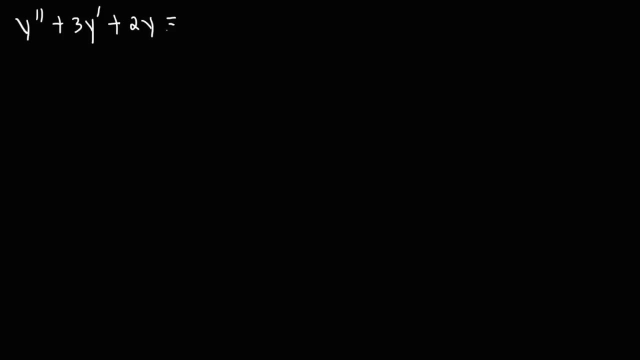 plus 2y, and this time we're going to set it equal to cosine x. So let's start with our homogenous differential equation. Let's make gx equal to 0.. So now, underneath that, let's write the auxiliary equation: ar squared plus br plus c is equal to 0.. 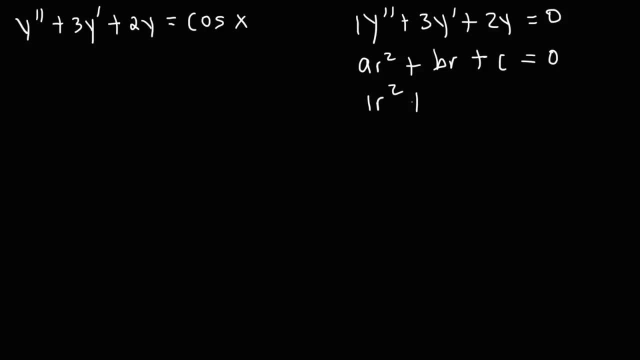 So we can see that a is 1,, b is 3, and c is 2.. Two numbers that multiply to 2 and add to 3 are 1 and 2.. So we have r plus 1 times r plus 2, and so we get two solutions. r is equal to negative 1,. 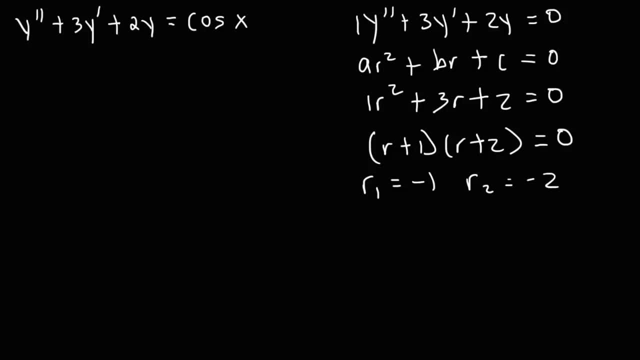 and r is equal to negative 2.. So, because we have two solutions, this is case number one of solving a homogenous differential equation, So our general solution will look like this: This is the formula that we're going to use. So, replaced in r1 and r2, we get that yc is c1, e to the negative x, plus c2, e to the negative 2x. 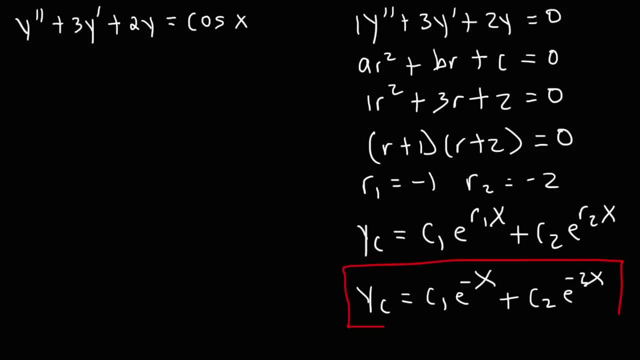 And let's save that equation. So now let's get rid of this stuff. So g of x, as we can see here, is cosine x. So we need to decide what we're going to write for y of p, The derivative of cosine is negative sine and the derivative of negative sine is positive cosine. 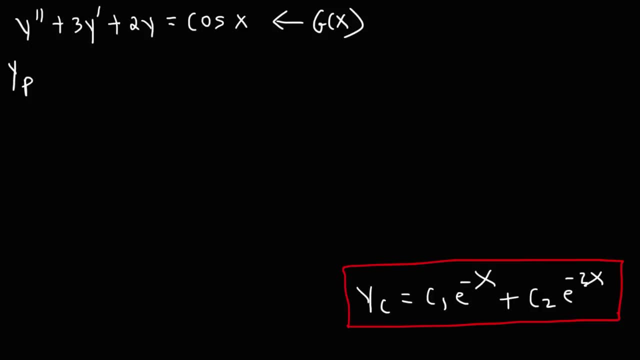 So yp must contain an expression with cosine and sine. So we're going to say that yp is equal to a cosine x plus b sine x. Now let's get the first derivative. So the derivative of cosine is negative sine. So we're going to have negative a sine of x. 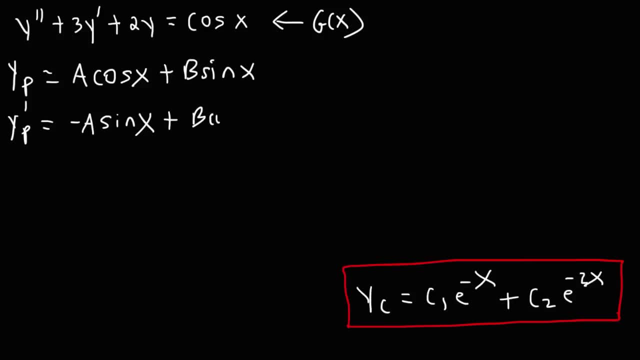 The derivative of positive sine is positive cosine. So this will give us b cosine x. Now let's move on to the second derivative. The derivative of negative sine is negative sine. The derivative of negative a sine x will be negative a cosine x. 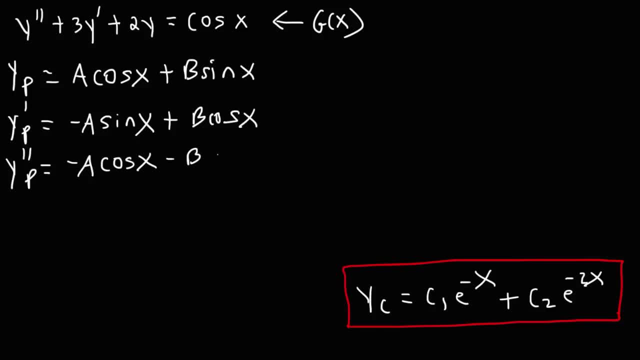 And the derivative of b cosine x is negative: b sine x. So now let's take this information and let's substitute it into that expression. By the way, write down this expression because I'm going to need the extra space, so I need to get rid of it for now. 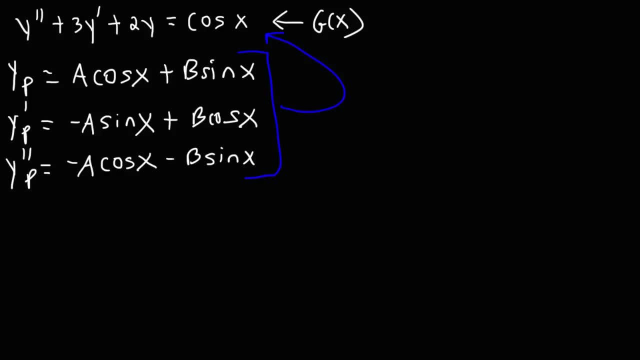 But just remember what it is, because we're going to use it later. So replace the negative sine x with negative b sine x. Now thisiesz the force of a negative sine x. So we'm going to replace this in y prime. I mean y double prime. 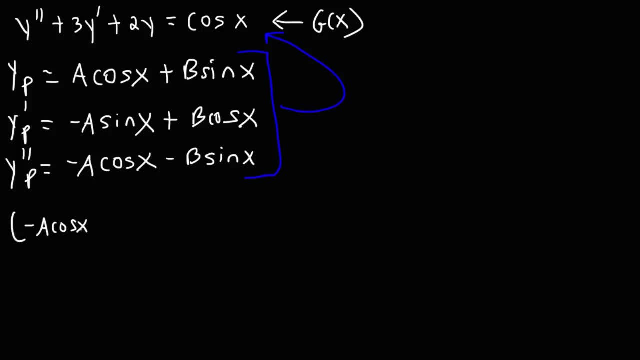 with negative a cosine x, minus b sine x, And then we have 3y prime. so that's going to be plus 3, times negative a sine x, plus b cosine x And then plus 2y, so 2 times a cosine b sine. 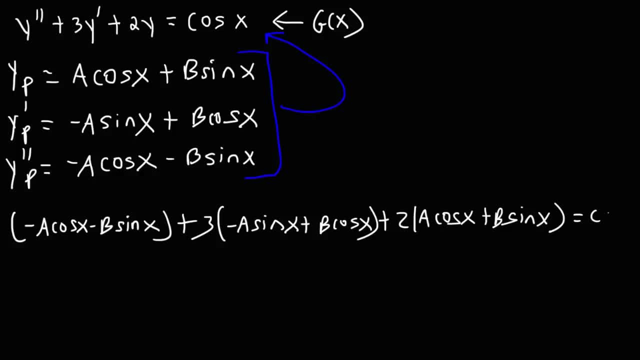 And all of this is going to equal equal cosine x. So let's combine like terms, Let's focus on the terms that have cosine. So this is negative: a cosine x plus 2a cosine x, So that becomes just 1a cosine x. 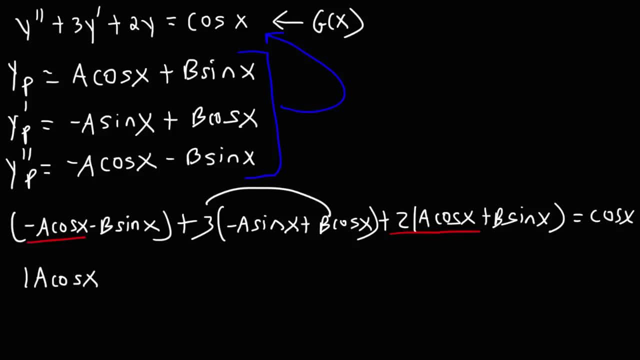 And then we have another cosine expression, That's 3b cosine x. Now let's focus on sine. So this is negative b sine x, and then 2b sine x. So that gives us positive b sine x, And then we have negative 3a sine x. This is going to be equal to 1 times. 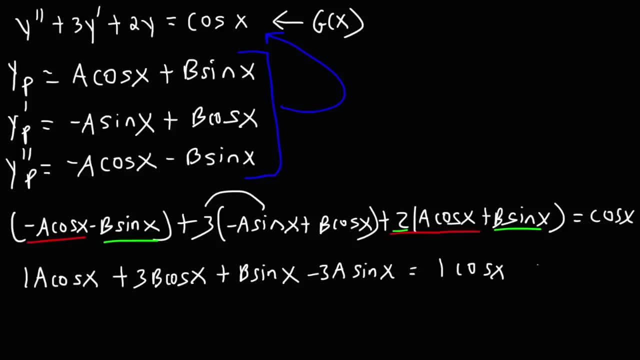 cosine x. We don't have a sine, but I'm going to write plus 0.. sine x. So let's gather all of the cosine expressions. Factoring out cosine, we're going to have a plus 3b is equal, or a plus 3b times cosine. And then, taking out sine, we're going to 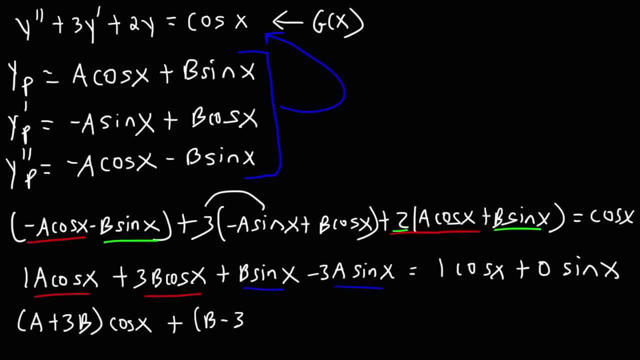 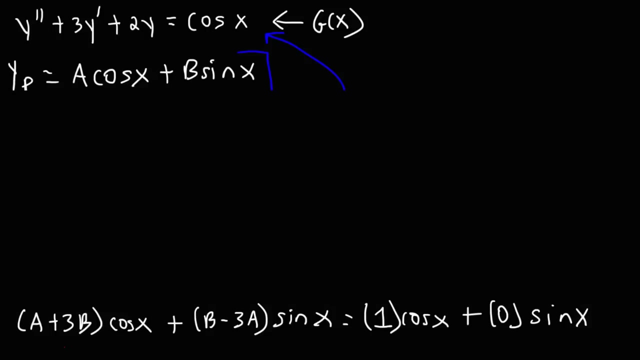 have b minus 3a times sine x, And so that's going to be 1 cosine x times cosine x plus 0 sine x. Now let's get rid of some of this stuff. So we could set 1 equal to a plus 3b. 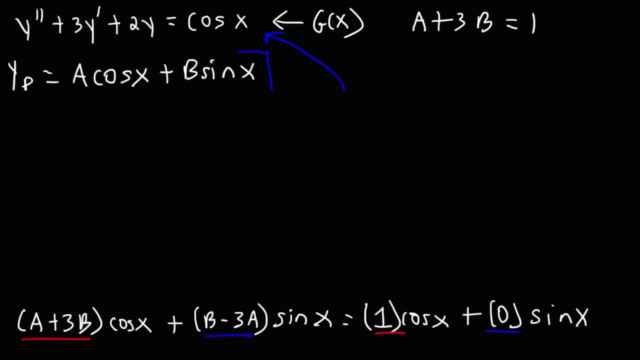 And we could set b minus 3a equal to 0. But I'm going to reverse the order, So I'm going to write negative 3a plus b. negative 3a plus b is equal to 0. So we need to solve by substitution or by elimination, rather. 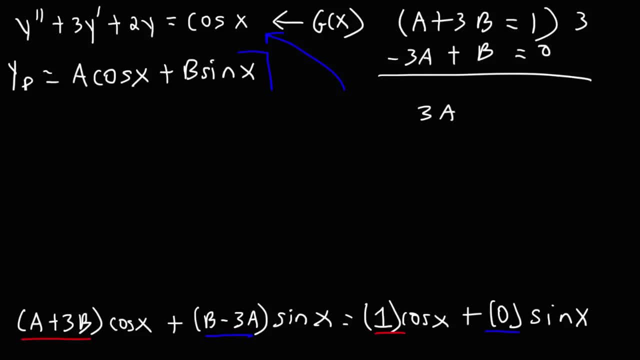 So I'm going to multiply the first equation by 3.. So it becomes 3a plus 9b is equal to 3.. And I'm going to rewrite the second equation the way it is And adding these two equations, we can cancel the a variable, So we'll get: 10b is equal to 3, which means b is 3 over 10.. 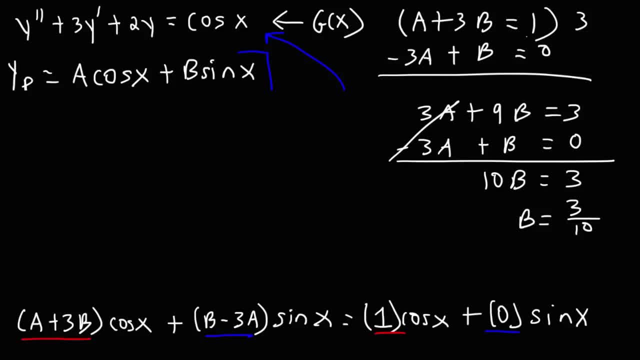 So now I'm going to use this equation to solve for a, So I have a plus 3b, or 3 times 3 over 10, equal to 1.. 3 times 3 is 9, so I get 9 over 10.. That should be a plus a. plus 9 over 10 is equal. 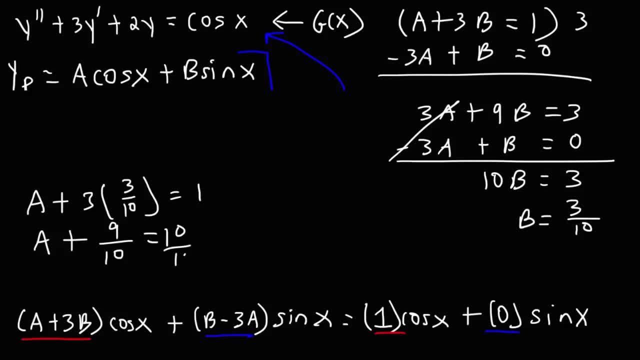 to 1.. So 1 is the same as 10 over 10.. Subtracting both sides by 9 over 10, we have 10 over 10 minus 9 over 10, which is 1 over 10.. So now we have the values of a and b, So we can plug that in into this expression to get yp. 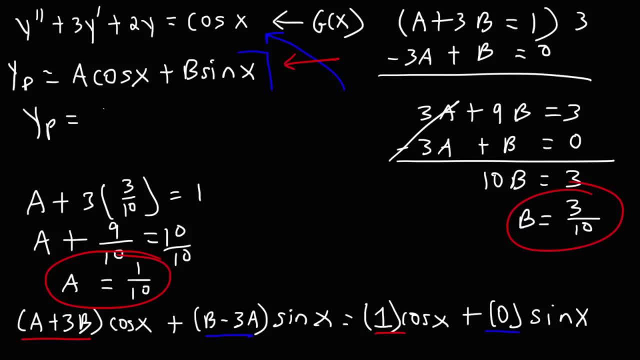 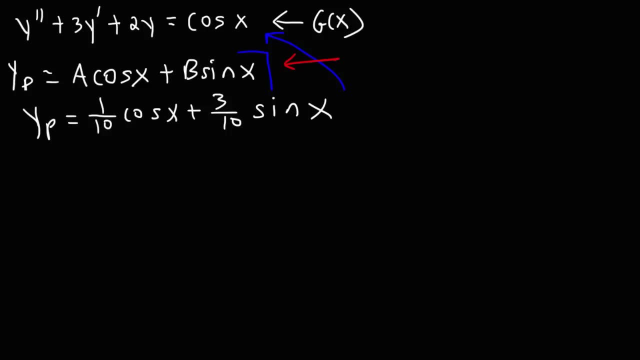 So we can say that y sub p is 1 over 10, cosine x plus 3 over 10 sine x. Now our next step is to factor out 1 over 10.. So we're going to have cosine x plus 3 sine x. And recall, we said that yc is equal to c1, e to the. 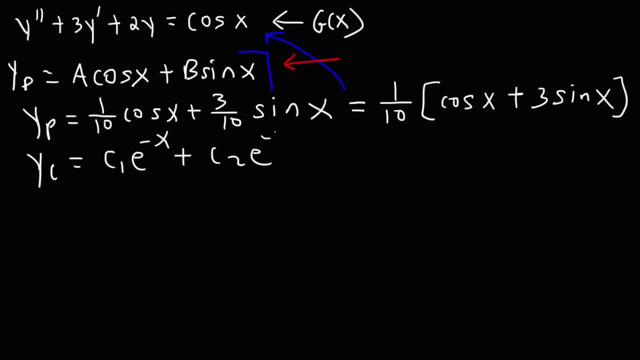 negative x plus c2 e to the minus 2x. So y is going to be the sum of yc plus yp. So the solution to our second order non-homogeneous differential equation is going to be negative x plus c2 e minus 2x plus 1 over 10, cosine x plus 3 sine x. 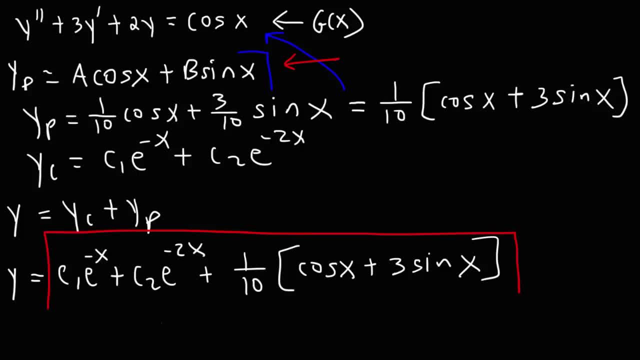 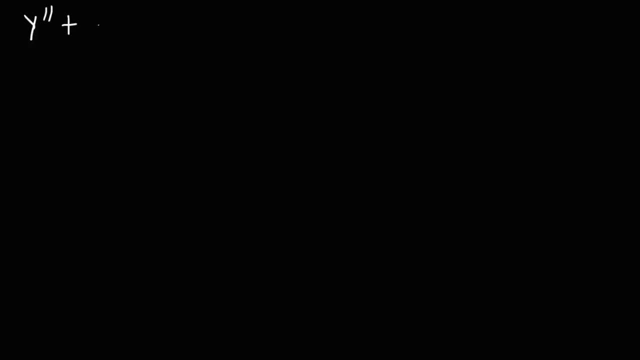 And so that's it for this example. For the next problem, let's try: y double prime plus y is equal to cosine. So, like before, we are going to start with our homogeneous equation. So we have y double prime plus 0. y prime plus y is equal to 0. 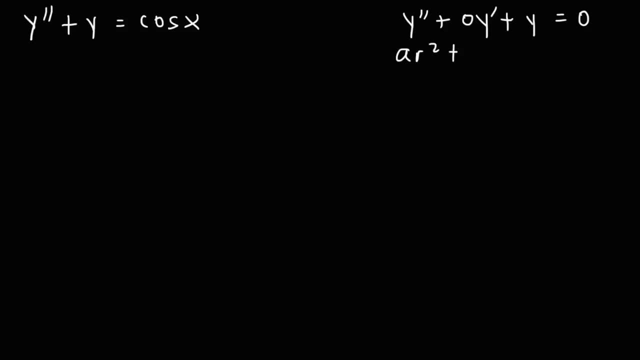 And then right in our auxiliary equation, right below it, we have this we could see: A is 1, b is zero, so that disappears and c is 1.. So r squared plus 1 is equal to 0, which means that r squared is equal to negative 1.. Taking the square root of both sides, we get: 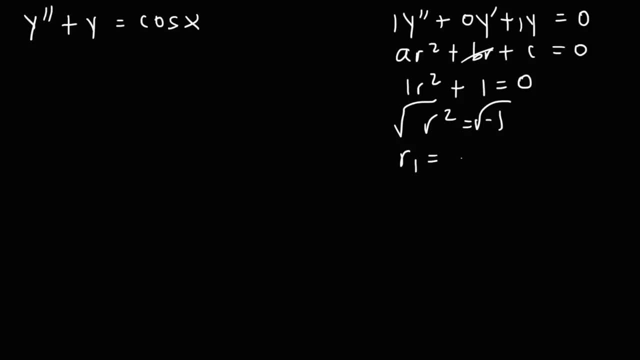 two imaginary or two complex solutions. So r1 is going to be 0 minus 1i, r2 is going to be 0 plus 1i. Now, the reason why I wrote it this way is so you can clearly see what alpha and beta are equal. 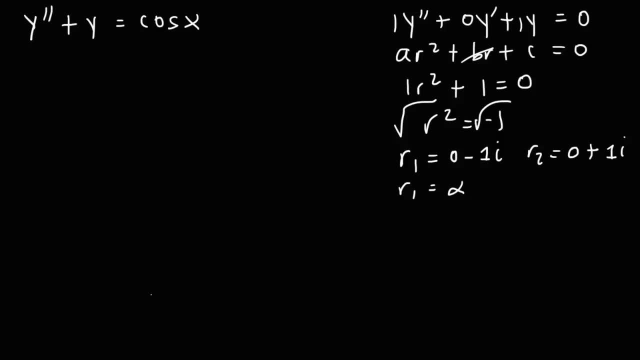 to. Well, this is going to be in the form alpha minus beta, and this one is alpha plus beta times i. Nevertheless, you can see that alpha is 0, beta is 1.. So the general solution for this homogenous equation is going to be e alpha x. 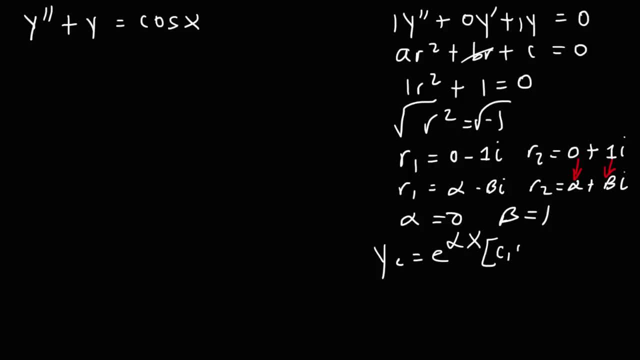 c1 cosine beta x plus c2 sine beta x. Alpha is 0, so e to the 0 is 1.. So we can get rid of that. Beta is 1.. So the general solution for this homogenous equation will be c1 cosine 1x plus c2 sine beta x, So we can get rid of that. 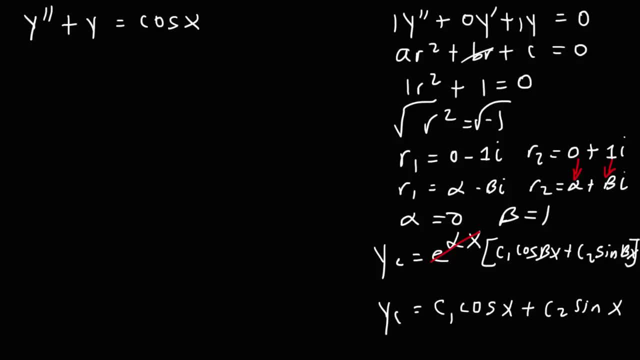 2 sine 1x, So let's save this for later. Now, g of x is cosine x, And typically for yp we would use a cosine x plus b sine x. However, for this example problem this is not going to be practical. 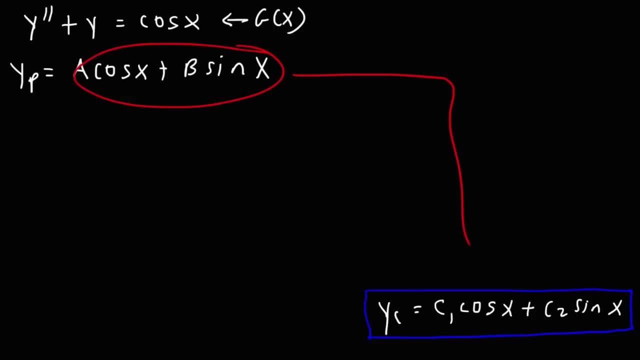 Because notice that this expression is the same as our complementary equation. So we don't want to use this expression, But let's see what would happen if we did use it. The first derivative it was going to be, the derivative of cosine, is negative sine. 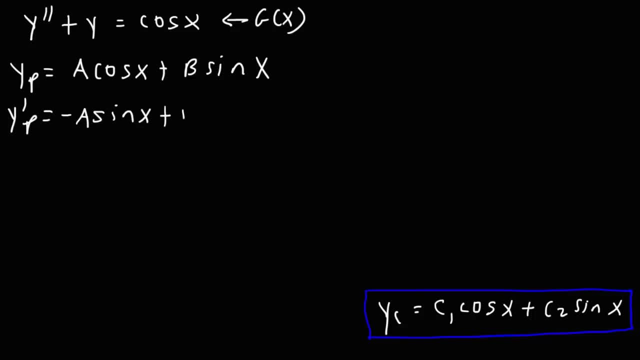 so we're going to have negative a sine x. The derivative of sine is cosine And then once we get the second derivative, it's going to be negative a cosine x And then b cosine will become negative b sine x. So if we were to plug in yp and y prime p, 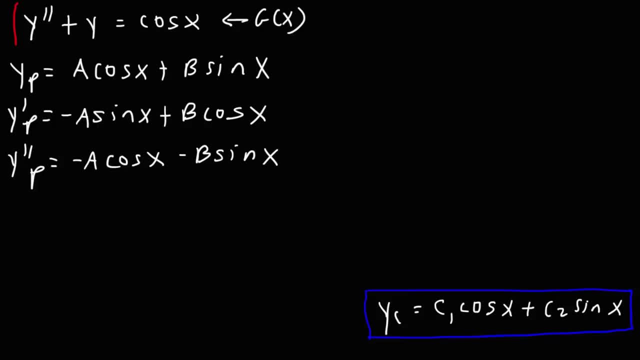 into this expression, that is y prime plus y. notice that a cosine x will cancel with negative a cosine x, b sine x will cancel with negative b sine x, And so in this example problem we will get zero equals cosine, which we can't do anything with that. 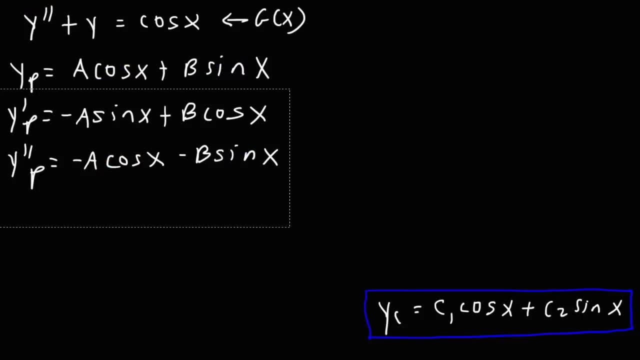 So this is not going to be practical, It's not going to work out very well. So, instead of using a cosine x plus b sine x, we're going to do something different: We're going to throw in an x variable into each term. 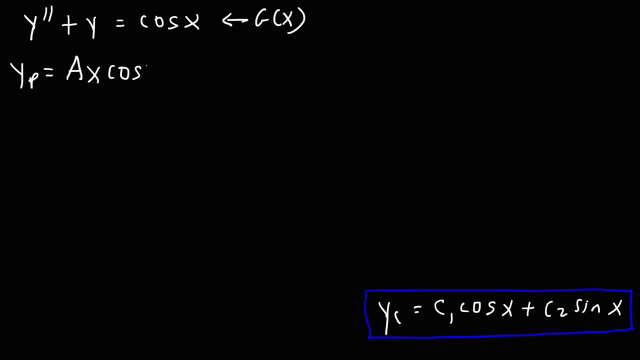 So instead of a cosine x, we're going to have ax cosine x. Instead of a, I mean b sine x, we're going to have bx sine x. So now let's get the first derivative. We need to use the product rule. 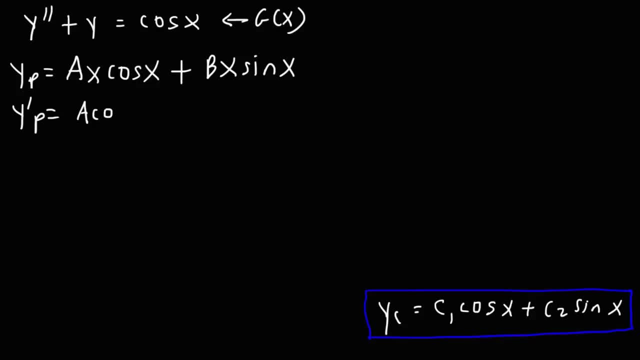 The derivative of x is 1, so we're going to get a cosine x. And then next we need to differentiate cosine x, which will give us negative sine x. So we'll have negative ax sine x. Moving on to the next term, 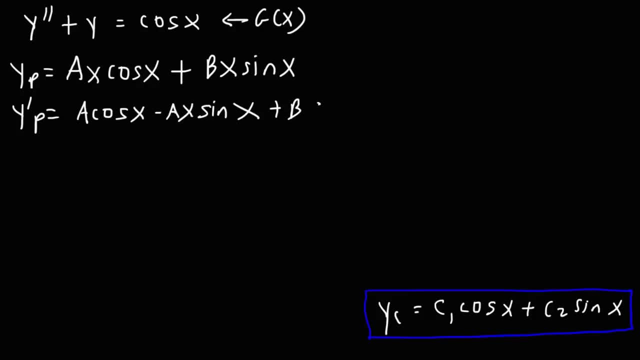 differentiating x will give us 1.. So we're going to get b sine x And then, taking the derivative of sine x, that's going to be cosine, positive cosine, So that's going to be bx cosine x. So now let's move on to the second derivative. 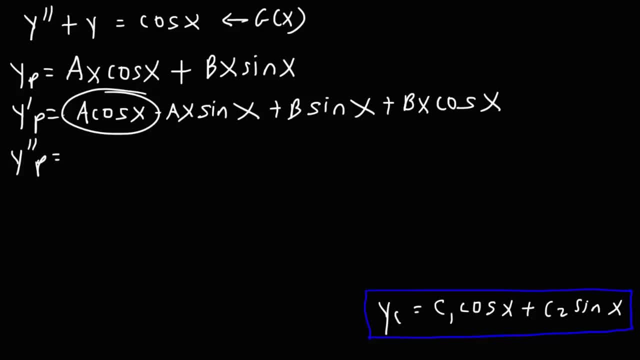 The derivative of a cosine x will be negative a sine x. Here we need to use the product rule. Differentiating x is 1, so that will leave behind negative a sine x. Differentiating positive sine will be cosine, and so we'll get negative ax cosine x. 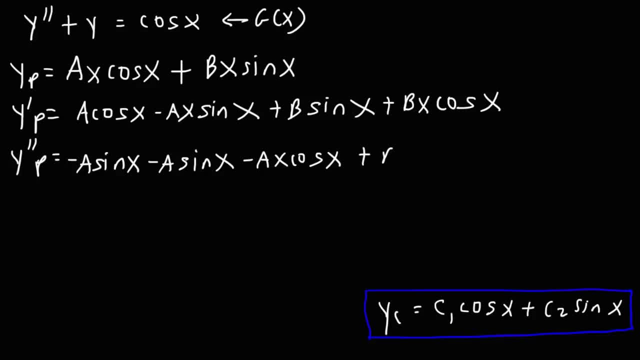 The derivative of b sine x will be b cosine x, And for this one we need to use the product rule again. So the derivative of a cosine x will be negative. ax- cosine x. differentiating x, we get b times 1 times cosine x. Differentiating cosine will give us negative. 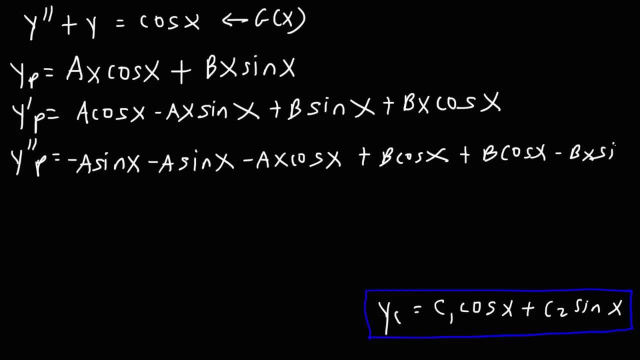 sine. So we'll have negative bx sine x. Now let's combine like terms. So we can combine these two terms. So that's going to be negative 2a sine x and then minus ax- cosine x. The next two terms that we can combine are those two, So plus 2b cosine x and then minus bx sine x. So now let's. 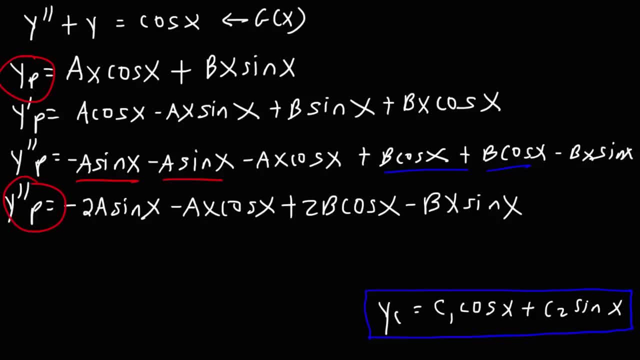 take yp and y double prime and plug it in into this expression. Now notice, once we plug in these two expressions into the left side of that equation, since we're adding y double prime and y, we could see that ax cosine x and negative ax cosine x will cancel, And then bx sine x and negative bx sine x will. 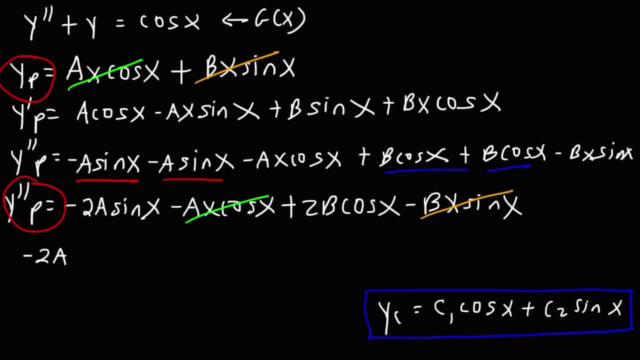 cancel. So that's going to leave behind negative 2a sine x plus 2b cosine x, And I'm going to put this in parentheses And that's equal to cosine x, But I'm going to write 0 times sine x, which is: 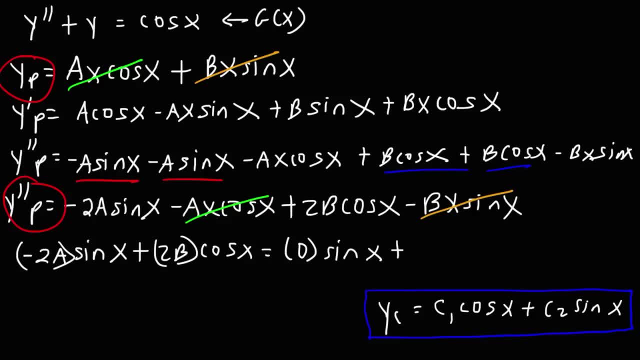 nothing plus cosine x, Or rather, let's say 1 times cosine x. So we can clearly see that negative 2a has to be equal to 0, because there is no sine on the right side. So if negative 2a is equal to 0, that means a is equal to 0. 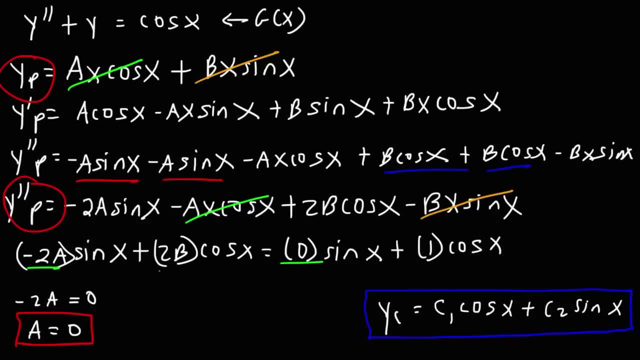 So this will be useful. Next, we have 2b equal to 1.. If 2b is equal to 1, b is going to be 1 half. So now, going back to yp, we want to plug in a and b into that expression, Since a is 0, this is going to disappear. 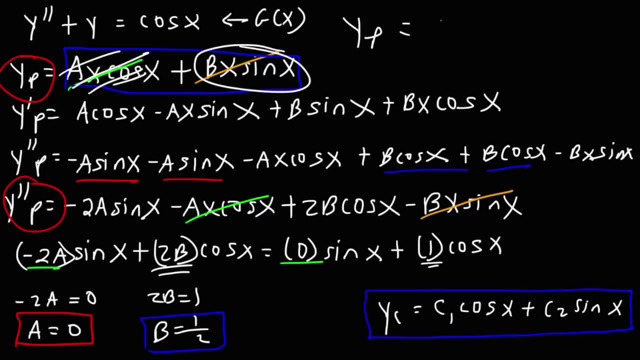 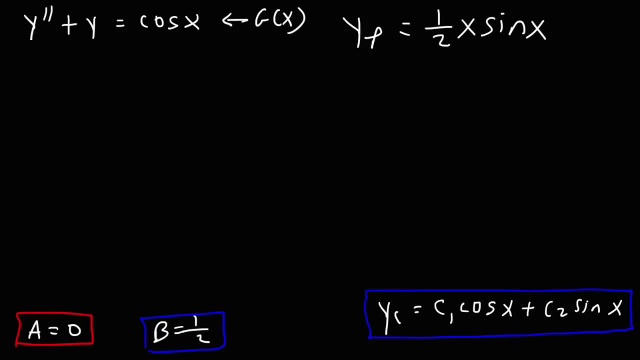 Now we can plug in b into that, because we have a number for b. So y sub p will be 1, half x sine x. So now that we have y sub p we can finish this problem. So our general solution: y, is going to be the sum of yc and yp. 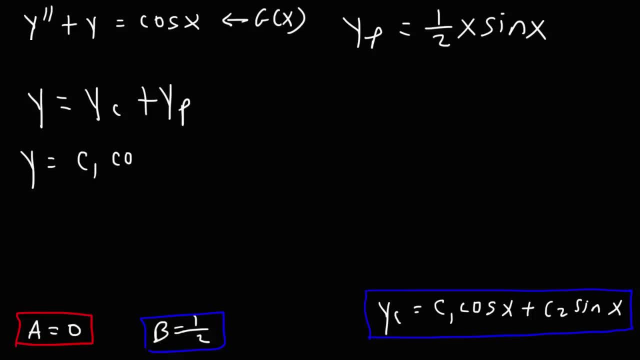 So yc, we know that's c1 cosine x plus c2 sine x. y sub p is going to be plus 1 half x sine x. So this is the solution to the differential equation. So that's the final answer for this example. 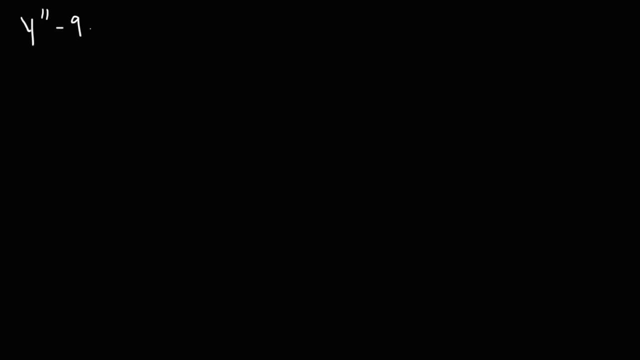 Now this is going to be the last problem. So here we have y, double prime minus 9y is equal to x, e to the x plus sine 2x. Go ahead and try that problem Now. as always, we are going to start with the complementary equation. 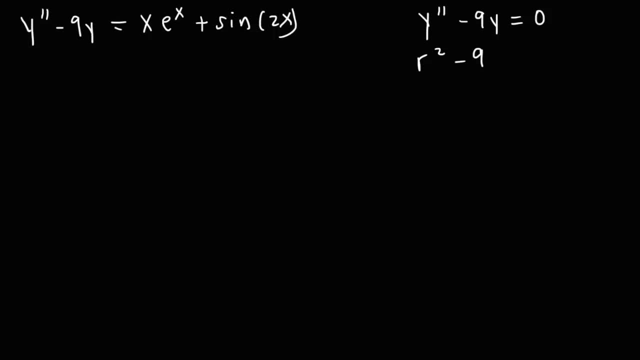 So we have: r squared minus 9 is equal to 0.. So that means r squared is equal to 9.. Taking the square root of both sides we get r is plus or minus 3.. So we have two real solutions. Thus we have case number one, where the general solution is going to be c1 e r1 x plus c2 e r2 x. 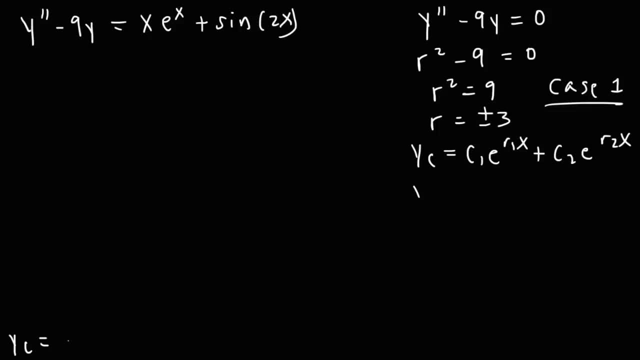 So let's write the solution here. So r1 is positive 3. And r2 is positive 3. And r2 is negative 3. So that's yc. We'll save this for later. Now notice that this problem that is on the right side contains a sum of two parts. 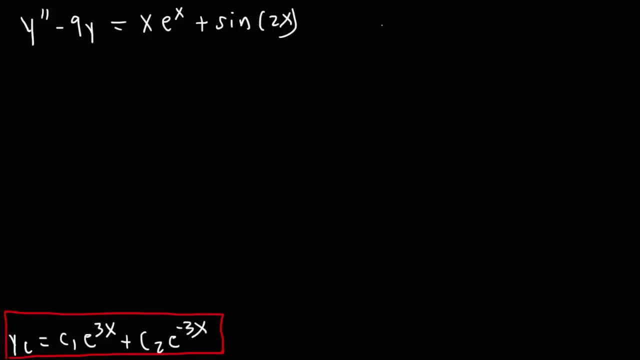 So to get the general solution to this differential equation, it's going to be y, which is equal to yc plus yp1 plus yp2.. yp2.. So yp1 will be associated with x, e to the x, yp2 will be associated with sine 2x. 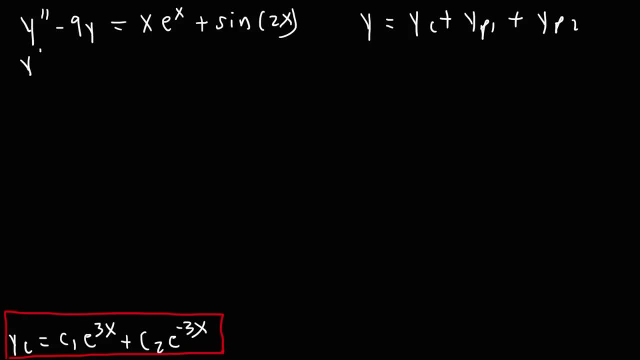 So let's focus on yp1.. So we're going to have y double prime minus 9y. We're going to set that equal to x, e to the x. Now, x is a linear expression And if you think of the straight line equation, y equals mx plus b. 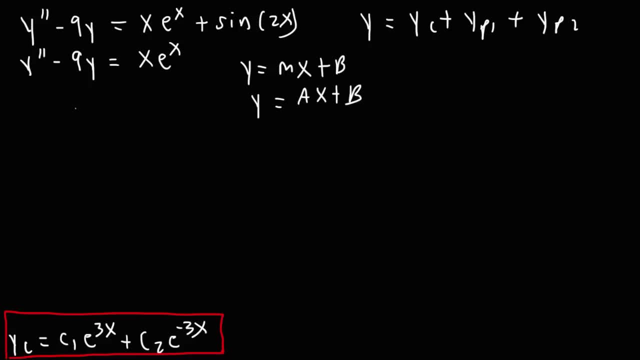 Instead of m we're going to use a, So for yp it's going to be ax plus b times e to the x. This is for the linear part of that expression. Now what we need to do is find the first derivative. 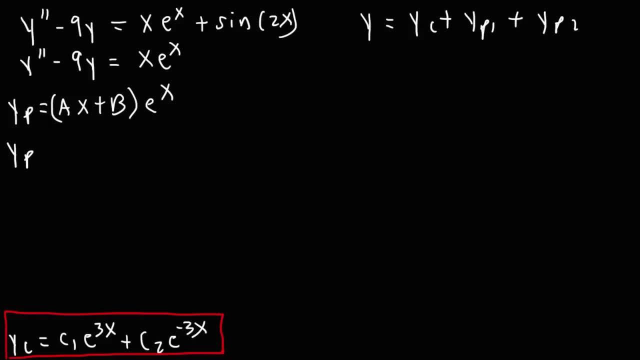 And we need to use the product rule to do that. The derivative of the first part, ax plus b, is simply a, And we're going to leave the second part alone. Next, we're going to Keep the first part the same. 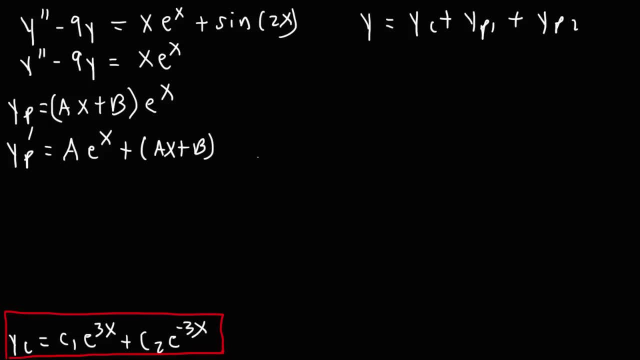 And then differentiate the second part. The derivative of e to the x is simply e to the x. Now we need to find the second derivative. The derivative of a e to the x is just a to the e to the x, And then we have the derivative of this thing again, which we did it here. 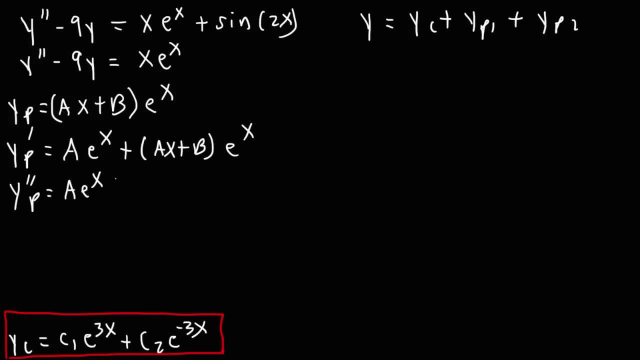 So we just got to rewrite this solution, So it's going to be plus a e to the x, plus a x plus b e to the x. So combining like terms, that is these two, we have 2a e to the x, plus a x plus b e to the x. 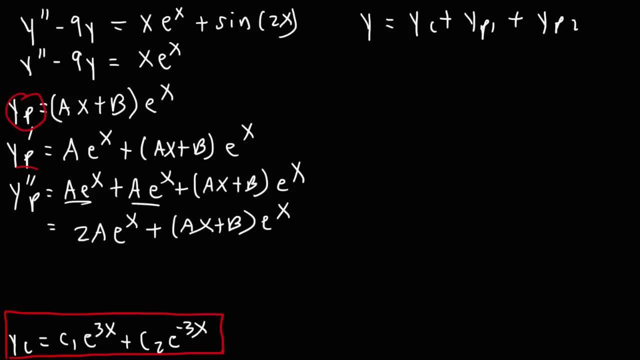 So now at this point we can plug in y and y double prime into that expression. So it's going to be what we have here: y double prime minus 9 times y And y is a x plus b times e to the x. 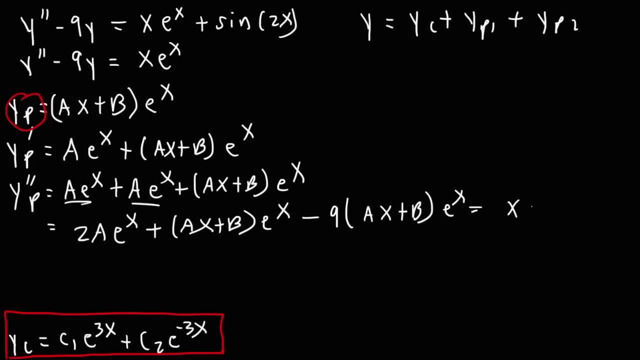 And that's going to equal what we have here: x, e to the x. Let's distribute and combine like terms. So we have 2a- e to the x, plus a x- e to the x if you distribute the e, And then plus b- e to the x. 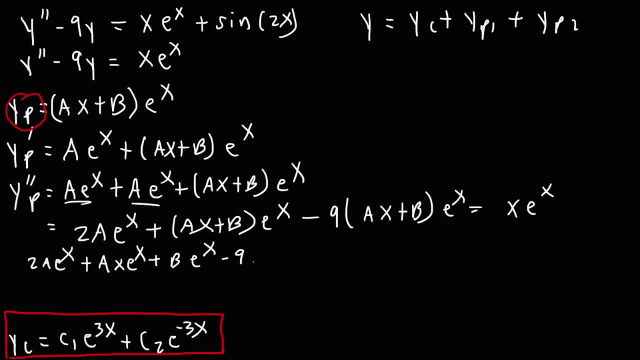 Distributing And then the negative 9, we're going to have negative 9a- x- e to the x And then negative 9b- e to the x, So we could combine these two. That will be negative 8a- x- e to the x. 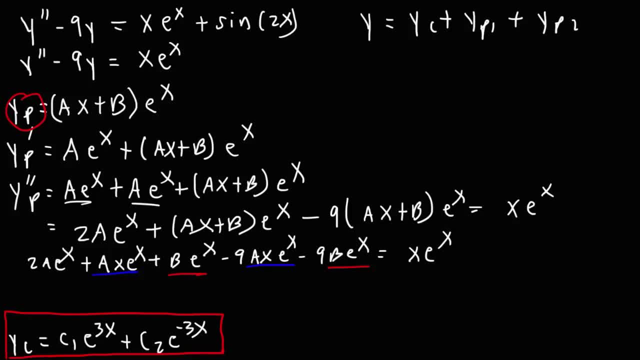 And we can combine those two, which will be negative 8b, e to the x. So we're going to have negative 8a- And I'm going to put that in parentheses- e to the x, And then combining all the constants. 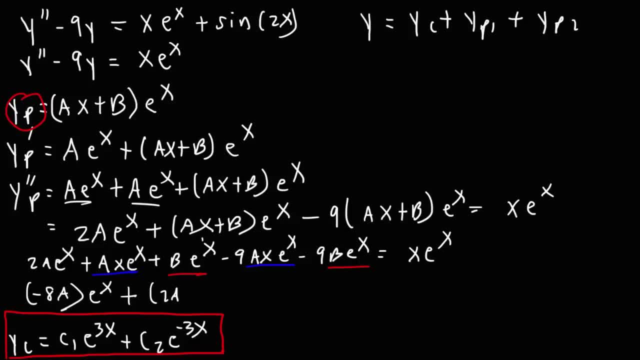 This one is 2a And these two combined that's negative 8b, And they're attached to e to the x Here. this is going to be 1 times x, e to the x. Oh, by the way, there should be an x here. 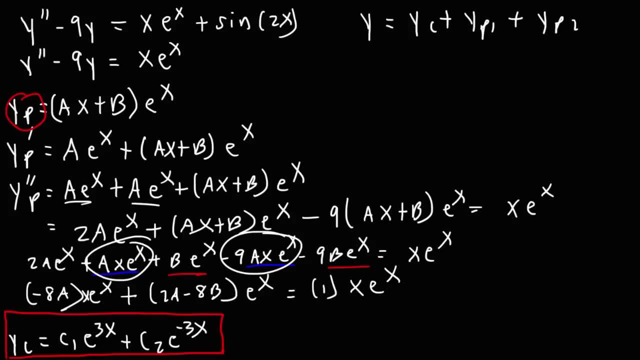 As we can see, this is negative 8a, x, e to the x, And then this has an e to the x, which we don't have on the right side, So I'm going to write that as 0 times e to the x. 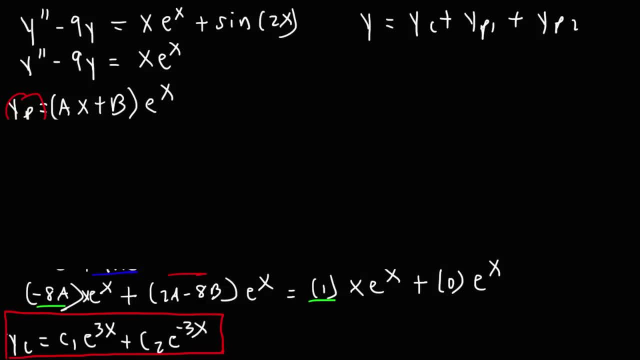 Now we're going to set negative 8a equal to 1.. So we can see that a is negative 1 over 8. And then we're going to set this equal to 0. So 2a minus 8b is equal to 0.. 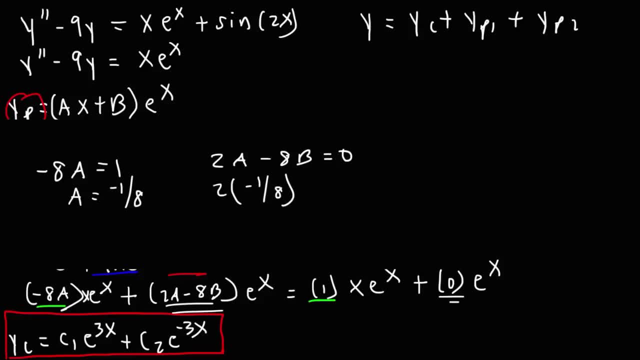 Substitute an a with negative 1 over 8. And then move in this to the other side. So this is going to equal positive 8b. Now, negative 1 over 8 times 2 is negative 1 over 4.. 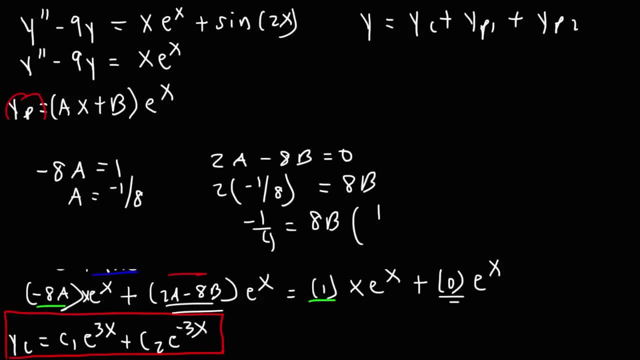 To get b by itself, we need to multiply both sides by 1 over 8.. So b is going to be negative, 1 over 32.. So now we could take a and b and plug it into this expression to get yp sub 1.. 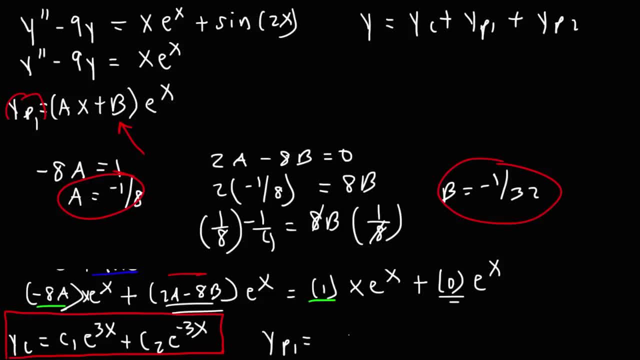 So yp sub 1, that's going to be- I'm going to factor out the negative sign from both of these numbers. So it's going to be negative 1 over 32.. So it's going to be negative 1 over 32.. 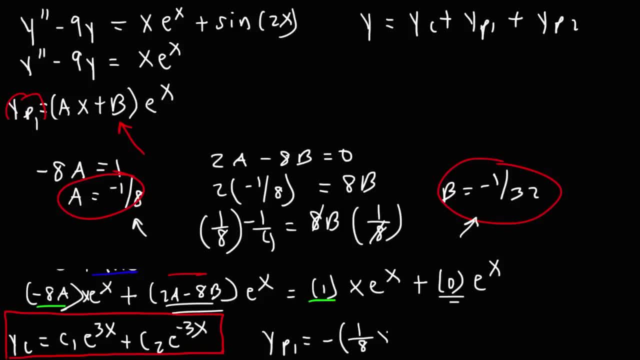 So it's going to be negative, and then 1 over 8x plus 1 over 32 times e to the x. So now that we have yp1,, we just need to get yp2, and then we can get our final answer. 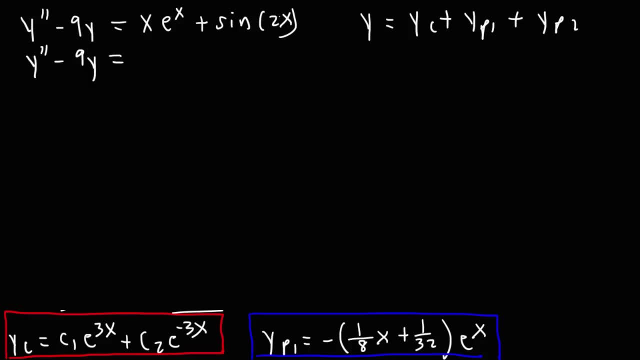 So we're going to set the left side of the equation equal to the second part of the right side of the equation, That is, sine 2x. So we need to decide what yp2 is going to be. So it has to have something with sine and cosine. 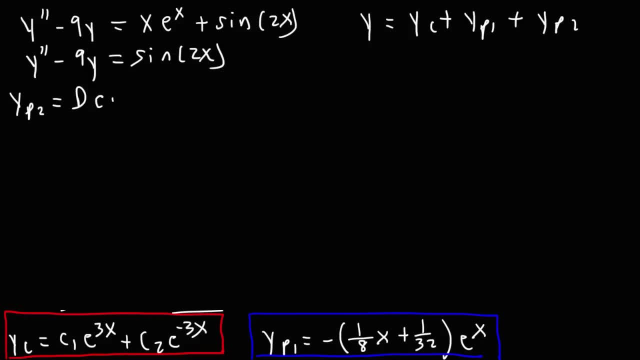 So we're going to set it equal to d cosine 2x and then plus e sine 2x. So now let's find the first derivative. The derivative of cosine x is negative sine x. The derivative of cosine 2x is negative sine 2x times the derivative of 2x, which is 2.. 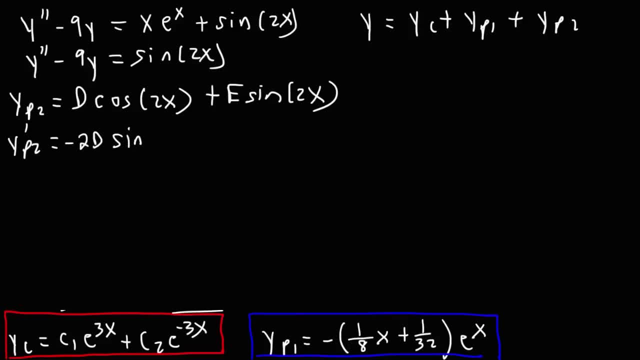 So we're going to get negative 2d sine 2x. The derivative of e sine 2x is going to be 2e cosine 2x. So now let's get the second derivative. So this is going to be the derivative of sine 2x. 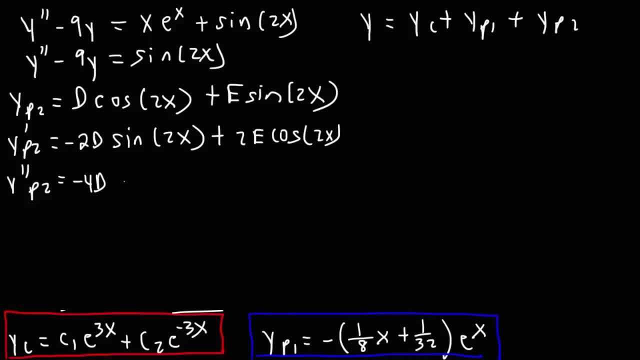 This is cosine 2x times 2.. So we're going to have negative 4d times cosine 2x And differentiating cosine 2x, we're going to get negative sine 2x times 2.. So 2e times 2, that's 4e, but with a negative sine. 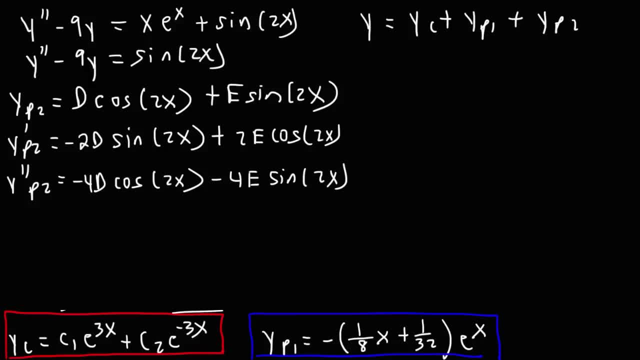 And then sine 2x. So now we have everything that we need, And so let's plug it into that expression. So y double prime, that's going to be negative: 4d cosine 2x Minus 4e sine 2x. 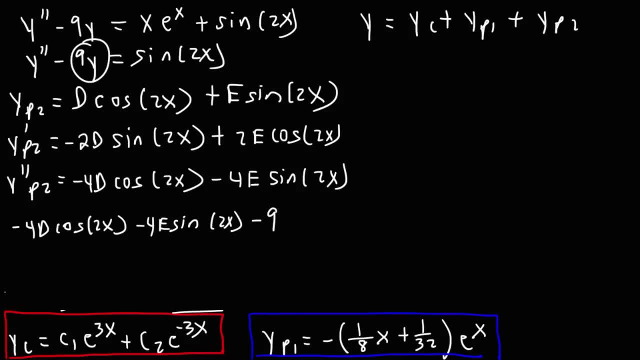 And then it's going to be minus 9y. So y is what we have here, And so that's d cosine 2x plus e sine 2x, And then that's going to equal sine 2x. So let's go ahead and combine like terms.